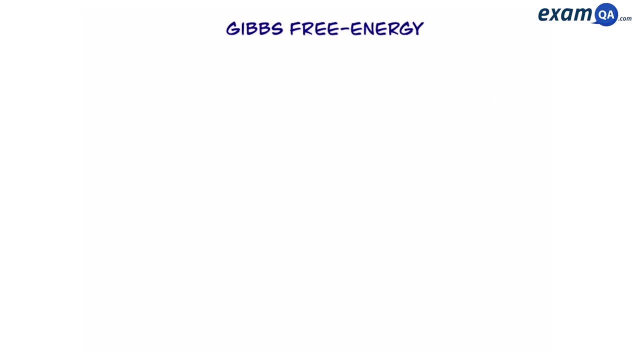 Welcome. In this video we're going to be learning about Gibbs free energy. So let's say we have this reaction: A plus B makes C and D. We want to know if this reaction will happen at 25 degrees Celsius. Now we have two options: It either will happen or it won't. 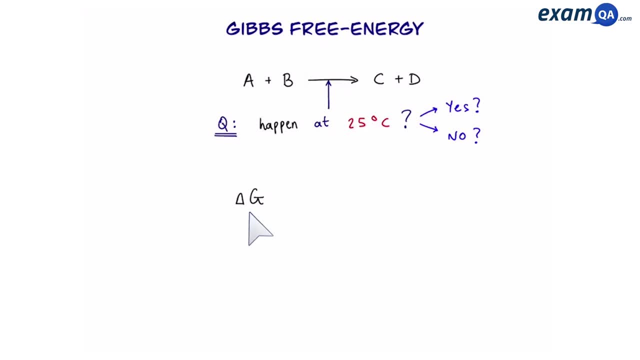 But to get to the answer we have to work out delta G. The G stands for Gibbs: free energy. If the value for delta G is negative, that means the reaction will happen. Another way of saying it will happen is to say it is feasible or is spontaneous. 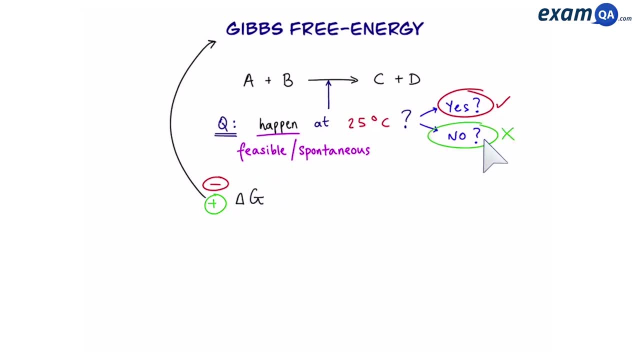 And if delta G is positive, then the reaction won't happen. So to work out delta G, we're going to use the equation delta H minus T, delta S. Now, before we continue, make sure you're familiar with calculating entropy changes. Okay, now we know. the units for delta H are kilojoules per mole. 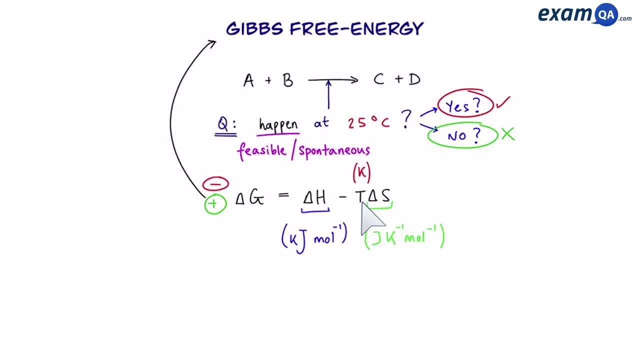 and temperature is measured in Kelvin. for this unit, Delta S stands for entropy, and it's measured in joules per Kelvin per mole. Now, since the units for delta G are commonly kilojoules per mole, that means we have to divide this by a thousand to turn the joules into kilojoules. 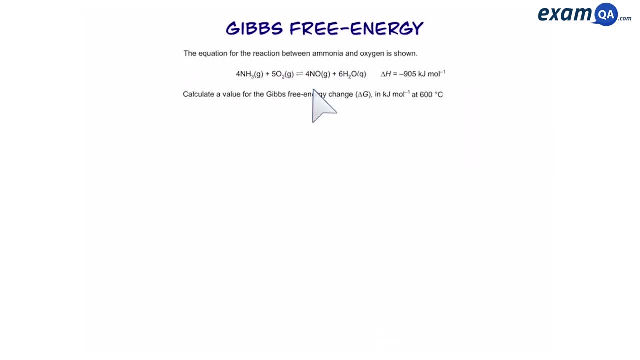 So here's an example of a question: Calculate the value for delta G. And we've also been given entropy data. So to work out delta G, we're going to do delta H minus T, delta S. We've already been given the value for delta H and temperature is given to us. 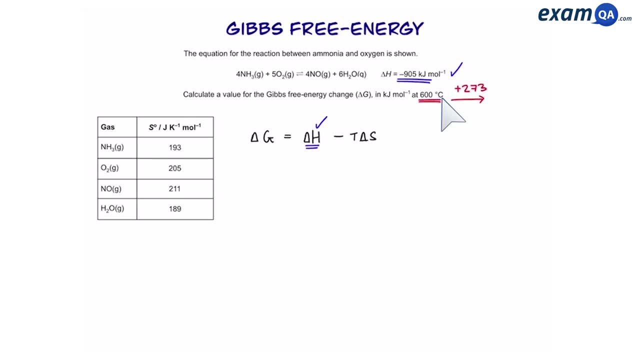 However, it's in degrees Celsius, So we're going to add 273 and turn that into Kelvin. Perfect. Now we also have the temperature To work out delta S. we haven't been given it, so we're going to use the data and use this equation to work out the value for delta S. 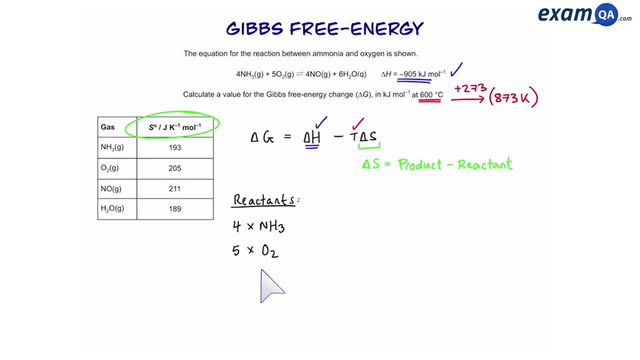 So reactants first, We're going to do four times ammonia and five times oxygen. So using this equation, The table, we're going to then add them together and that gives us 1797.. That's the total entropy of the reactants. 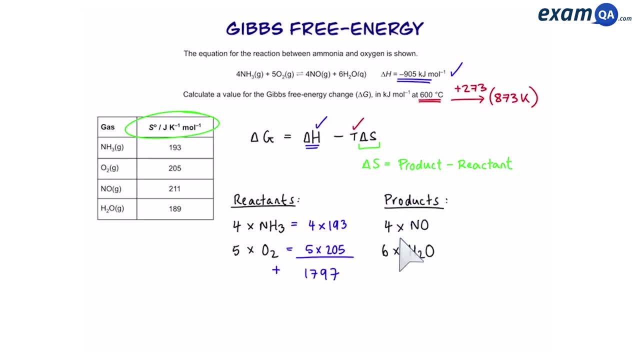 We're going to do the same for the products. So four molecules of nitrogen monoxide and six water, And adding them together gives us one, nine, seven, eight. Next, we're going to do products: take away reactants and we get one, eight one. 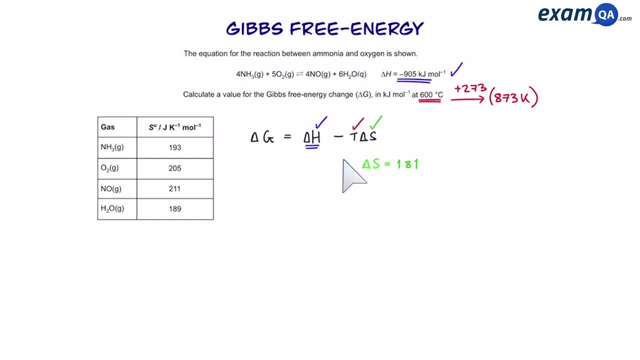 So now we have all three components of the equation. Let's now plug them into the equation and work out the value for delta G Minus nine zero five for enthalpy: Minus nine zero five for enthalpy. Take away temperature in Kelvin. 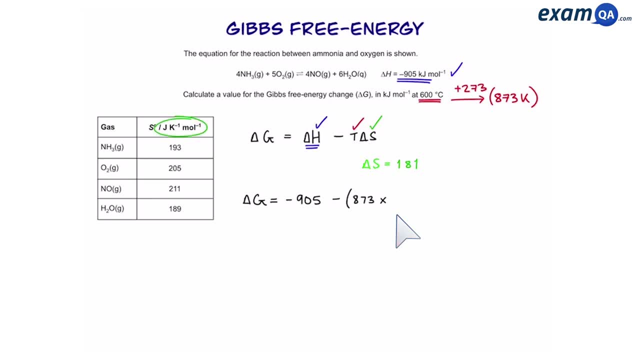 Time is by entropy. Now notice, the entropy has been given to us as joules, So we have to divide this by a thousand to turn it into kilojoules, And then we can put that into the equation, And that gives us an answer of minus one zero six three kilojoules per mole. 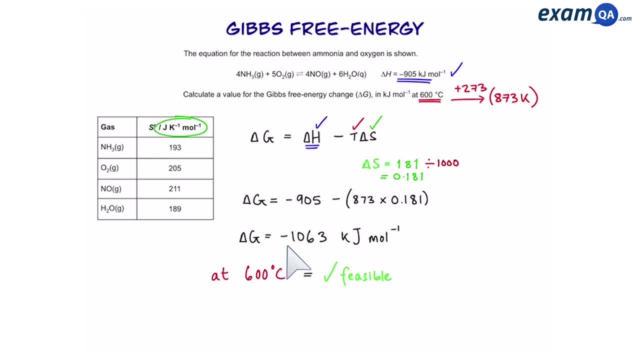 Also because it's a negative value. That means, at six hundred Degrees Celsius, This reaction is feasible. Now part B. Here's the next part of the question. The same reaction was carried out at a higher temperature. Explain how this would affect the value for delta G. 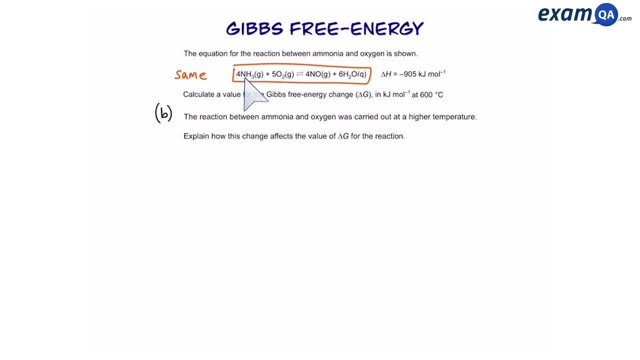 Since it's the same reaction, That means the entropy change will be the same And so will the enthalpy. However, the temperature has increased. So if we look at our equation, We can see that we have two main components: Delta H. 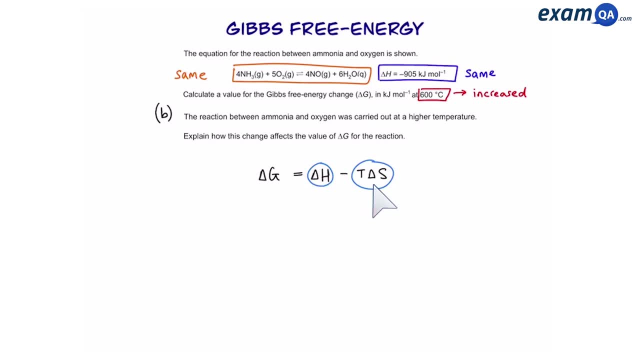 And T delta S. Delta H hasn't changed. However, T, Which is part of this component, Has increased. Therefore the whole component becomes greater. So the value for T delta S becomes larger. This means now we have delta H, take away a larger number. 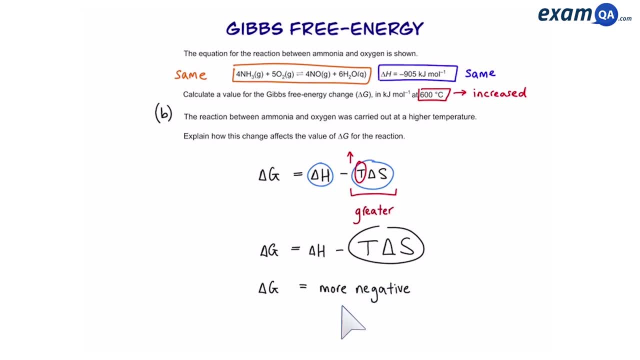 And as a result, the value becomes more negative. So here we saw that changes in temperature can affect the value for delta G. Next we'll look at how changes in enthalpy And temperature And entropy can affect delta G. So whenever you have a reaction, 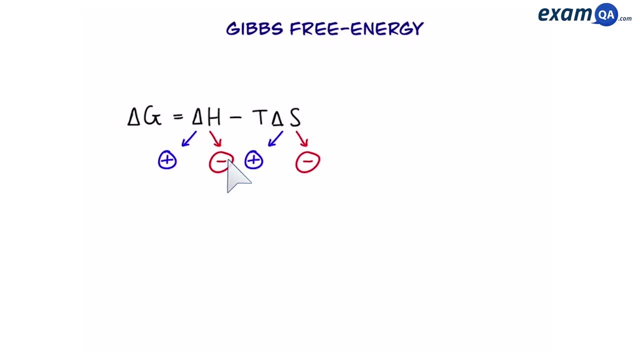 Enthalpy can be positive or negative, And so can entropy. Temperature will always be a positive value Because it's measured in Kelvin. The lowest value for Kelvin is zero And from there it just goes up. So because we have two types of enthalpy. 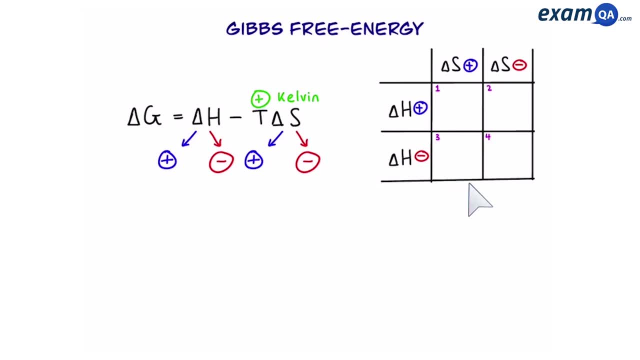 And two types of entropy, We can get four possible combinations. So let's look at all four scenarios And see how they affect delta G. We want to look for When will the reaction Be feasible, Ie When will delta G be negative? 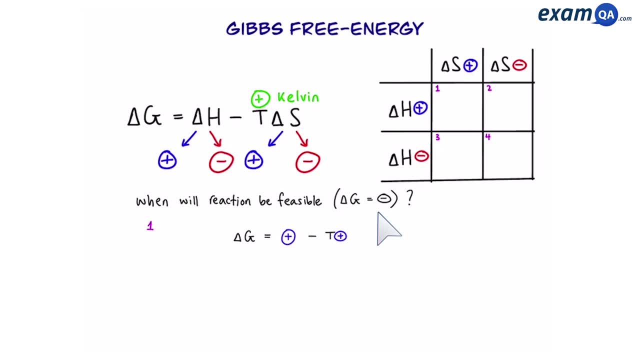 So let's start with scenario one. In scenario one, Delta H is positive And delta S is positive. That gives us A positive number. Take away temperature Times- a positive number. To make sense of this, We'll use some random numbers. 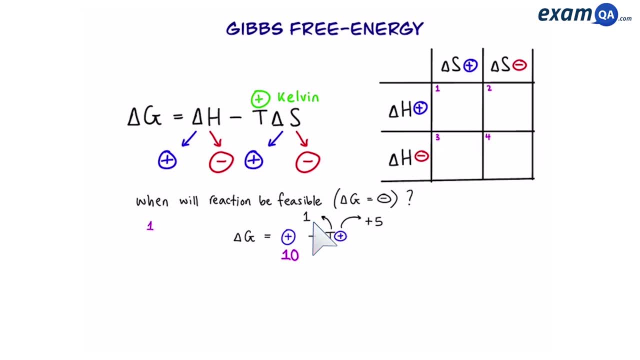 So let's say enthalpy is plus ten, Temperature is one And entropy is plus five. That means Together these two will become One times five, Which is five, And the equation becomes Ten. take away five, Which gives us plus five. 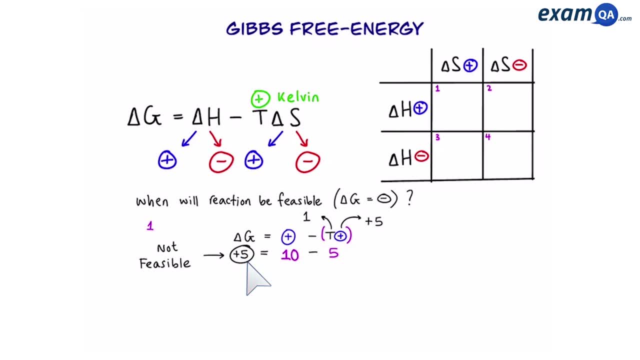 So that's a positive number, Meaning the reaction will not be feasible. However, What about when temperature is large, When temperature increases? So let's say, instead of one It becomes ten. Now things become a bit different. We still have a positive number. 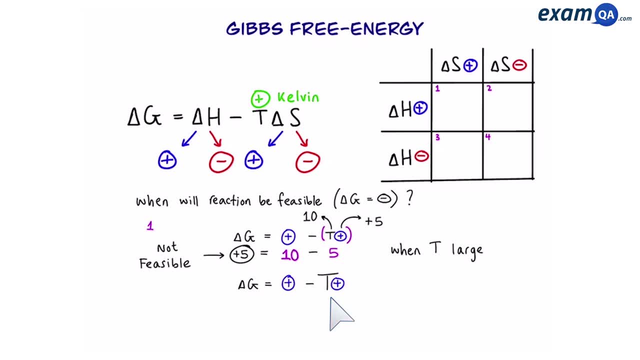 Take away a positive number. However, because temperature is larger, That means we have a greater value For T delta S. So now we have ten. Take away fifty, Which gives us minus forty five, And that makes it feasible. So to summarise: 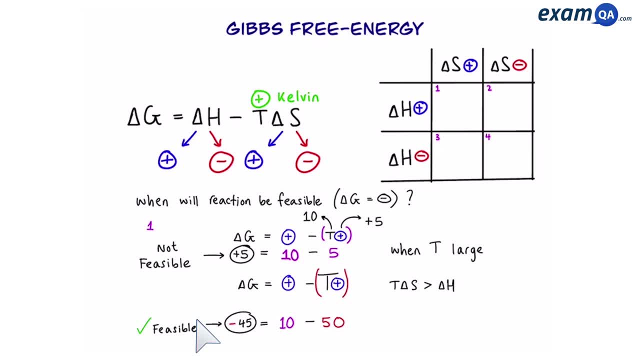 In the first scenario, When you have a positive delta H And a positive delta S, The reaction will only be feasible When temperature is high, Or in other words, When T delta S Is greater than delta H. Now we have a positive delta H. 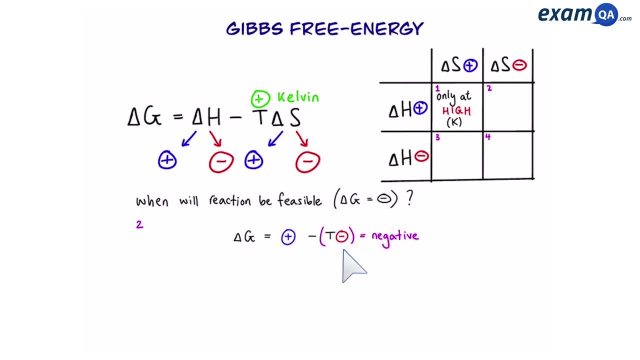 But a negative delta S. That means this part Will always be a negative value. So we have a positive value, Take away a negative value. And we know that plus, Take away minus Is going to be always positive, Since delta G will always be positive. 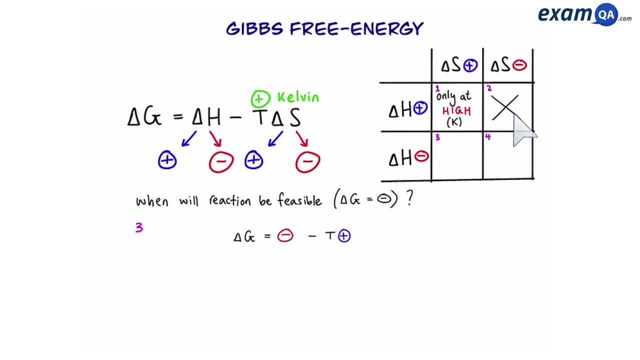 That means the reaction will never be feasible. Moving on to scenario three, Now we have a negative delta H And a positive delta S. This part, therefore, will always be a positive number. So we have a negative value. Take away a positive value. 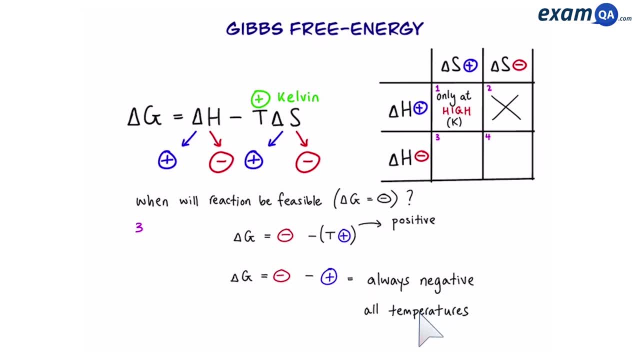 This will always be negative, So that means at all temperatures The reaction will be feasible. Moving on to the last one, So now we have a negative delta H And also a negative delta S, So we'll use some random numbers. Let's say that delta H is minus 10.. 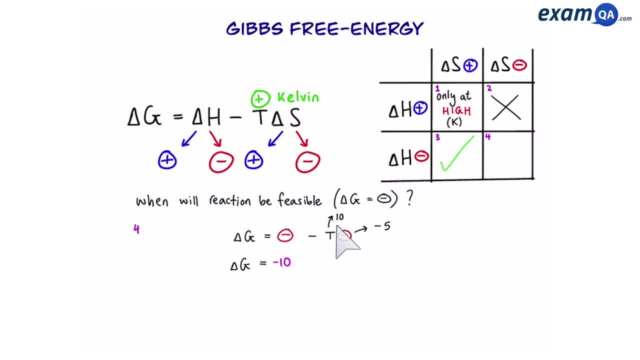 Because it's negative. Temperature is 10. And delta S is also going to be minus 5. Also a negative number. So that means 10 times minus 5. Will be minus 50. So we have 10. take away minus 50.. 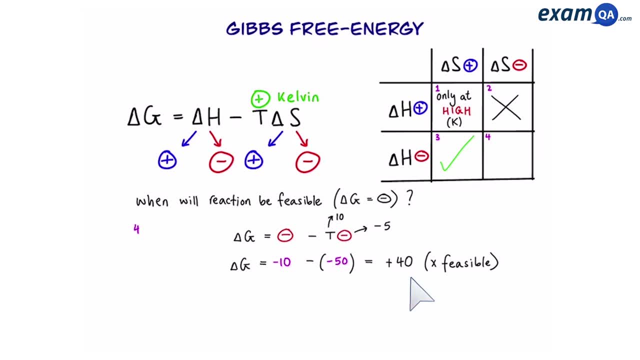 And that gives us plus 40. So, because it's positive, That means the reaction is not feasible. However, what about if we lower the temperature? So instead of 10. The temperature is now 1. That means we have 10, take away minus 5.. 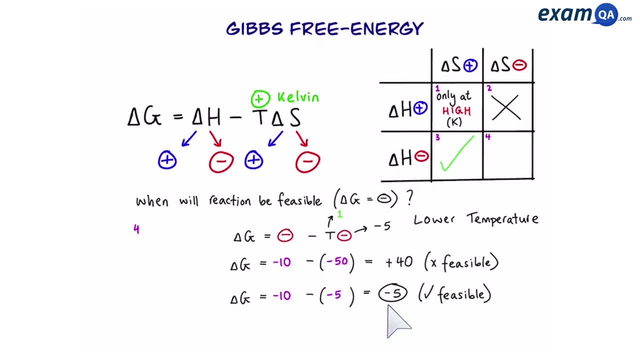 And this gives us minus 5. A negative answer. So that means the reaction will be feasible. So to summarise In scenario four, When both delta H and delta S Are negative, The only time the reaction will be feasible Is at low temperatures. 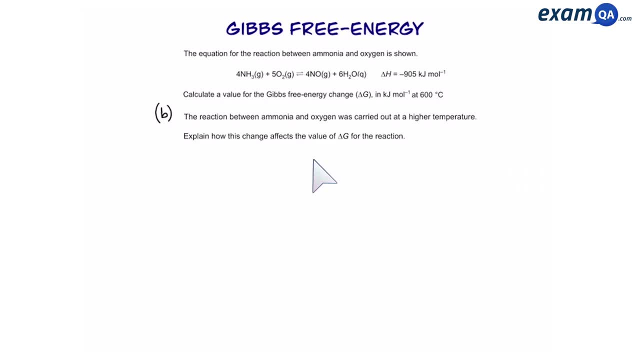 So, going back to this question again, Let's see if we can answer it Using what we've learnt. So we've been given the data already And we can use our table that we just made, And so we know that the reaction falls under this category. 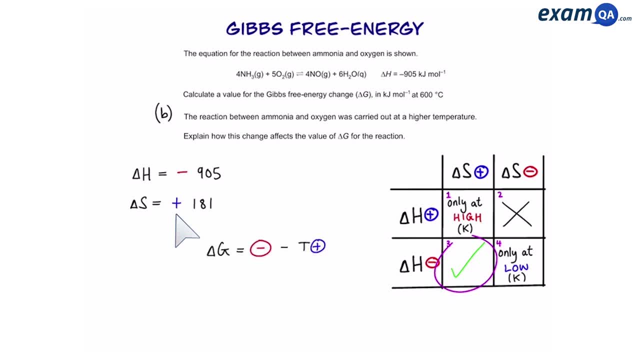 Delta H is negative And delta S is positive, So delta G is going to be equal to minus. Take away plus. However, The temperature has increased, As mentioned in the question, So if the temperature increases, That means all of this becomes larger. 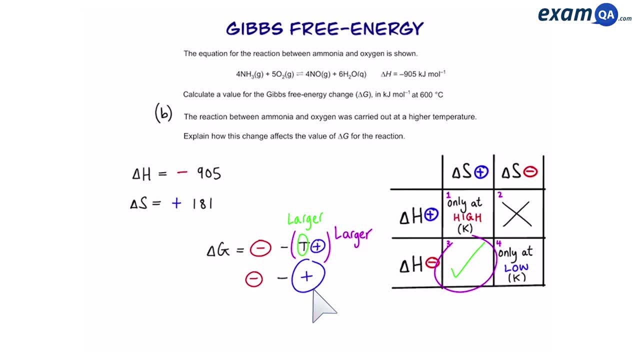 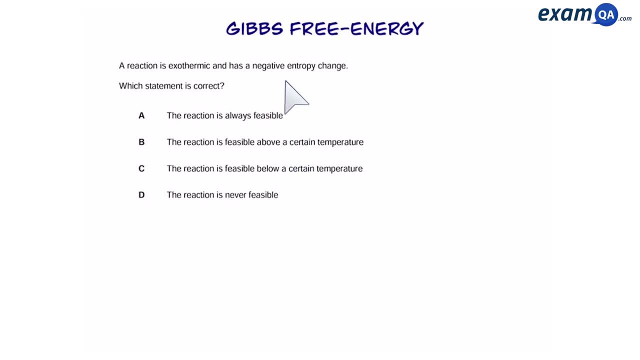 So now we have minus. Take away a larger number. Therefore it's going to be more negative. Okay, so here we have an example of a multiple choice question. To answer these kind of questions, It's very important to use your table. So the question says: 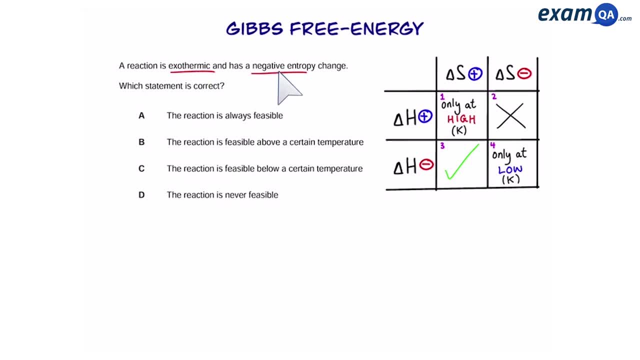 We have an exothermic reaction Which also has negative entropy. This falls under category four And therefore the answer is: The reaction will only be feasible Below a certain temperature. Okay, pause the video And see if you can try answering this one. 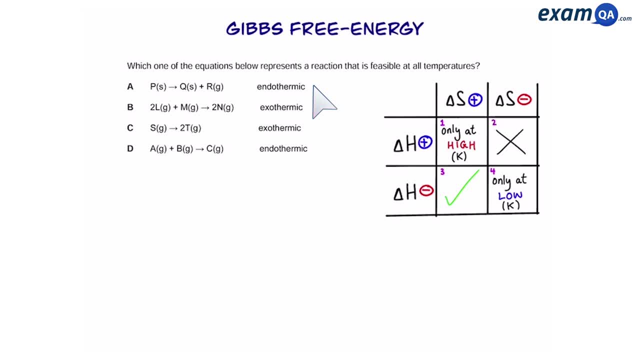 Which of the equations below represents a reaction That is feasible at all temperatures? With the table, It's very easy to see That we want something like this: Enthalpy to be negative And entropy to be positive. So let's go through each of these.